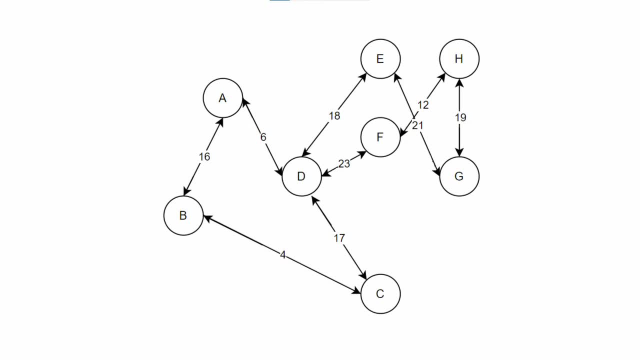 find the most efficient path to help the tired postman. This problem can be represented with a graph that includes edges and vertices. In this case, the neighborhood would be the graph, each intersection would be a vertex and each street would be an edge, with the houses lining the streets. 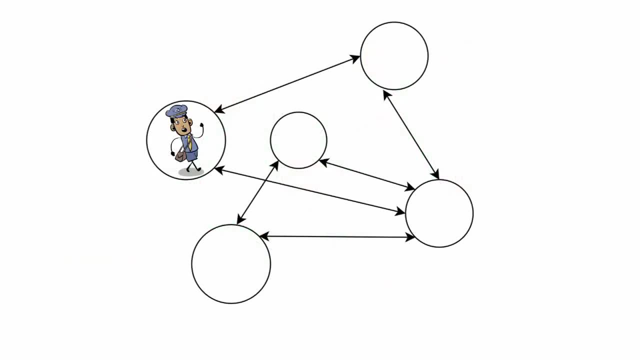 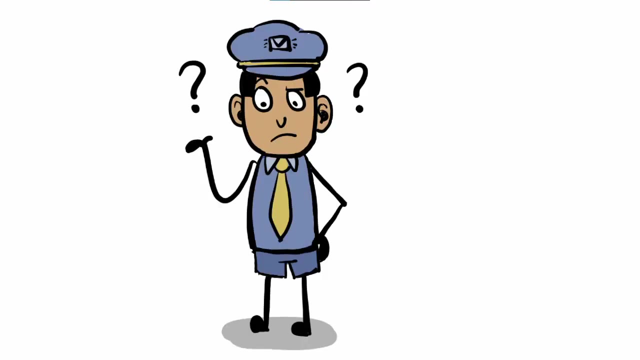 The ideal scenario for a postman would be to travel each street exactly once before returning to the post office. If we can traverse every edge exactly once and finish at the starting vertex, we would have what's known as an Eulerian graph. But how do we figure out if a graph is Eulerian without just guessing and checking? 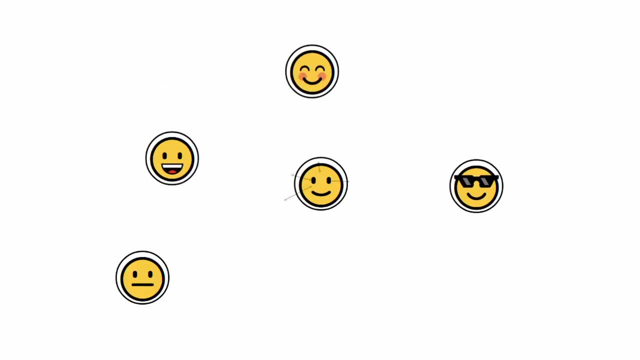 Well, first we have to figure out what's known as an Eulerian graph, and then we have to look at the degree of each vertex, which is the number of edges attached to a specific vertex. If the graph has vertices that are all of even degree, the graph is Eulerian. 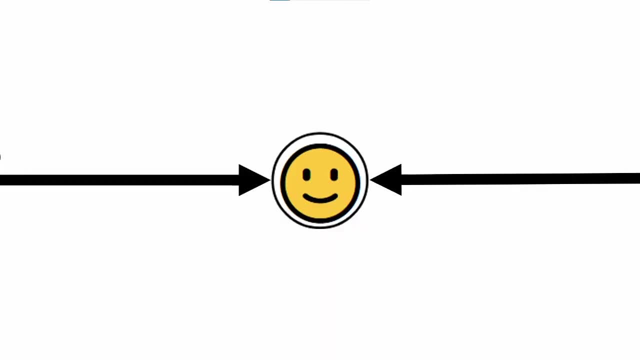 That works, but why? Well, if you have a vertex of degree 2, then you have two edges connecting to that vertex, one edge to go in and one edge to go out. Therefore, if you have an even number of edges connecting to an intersection, then you have two edges connecting to that vertex- one edge. 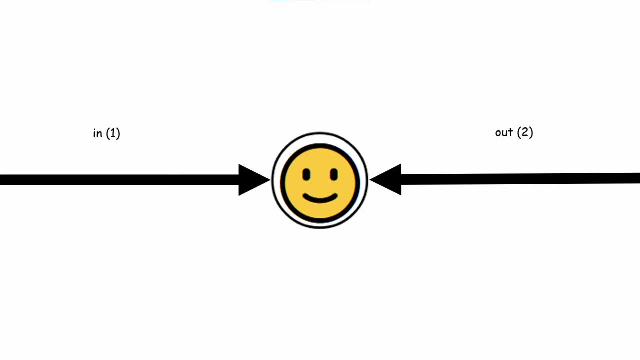 to go in and one edge to go out. In other words, if you have an even number of edges connecting to an intersection, you never have to travel an edge twice to pass through that intersection. However, If you have a vertex of odd degree, then you have a way to reach. 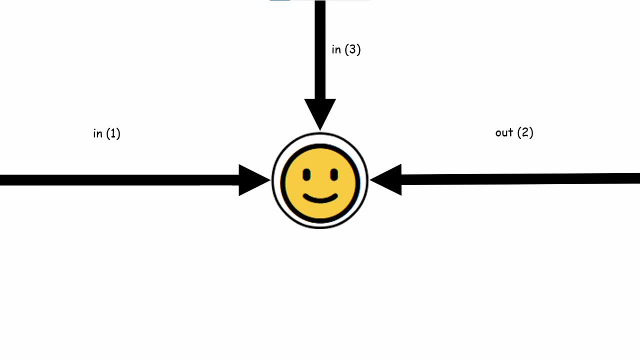 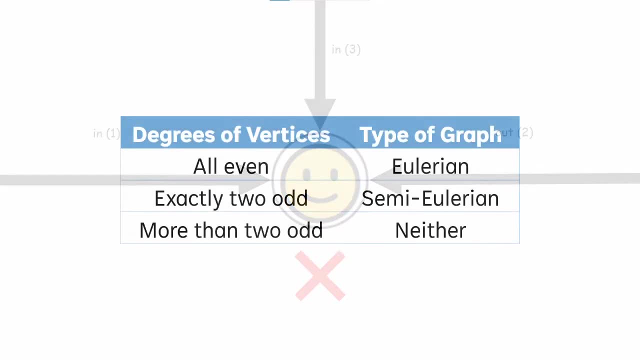 the intersection, but no way to leave it without traveling along one of the connected streets twice. If the graph has exactly two vertices of odd degree, the graph is Semi-Eulerian. Semi-Eulerian graphs are similar in that you can traverse every edge once, but different in that you. 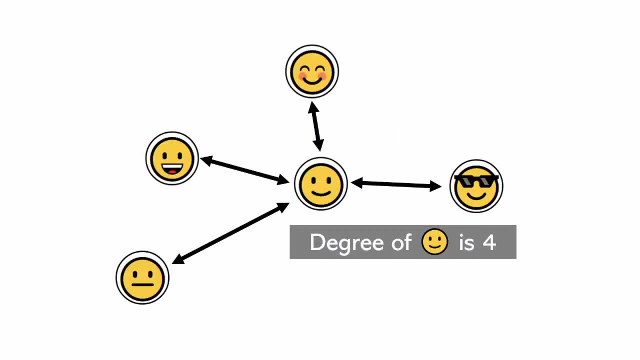 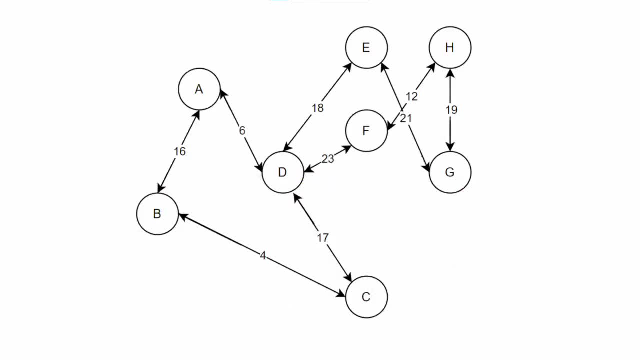 cannot start and finish at the same vertex, And if the graph doesn't finish at the end fit either criteria, then it's just a regular graph. It's not Eulerian at all. Oh, I see, If the neighborhood could be represented by an Eulerian graph, that would be fabulous. 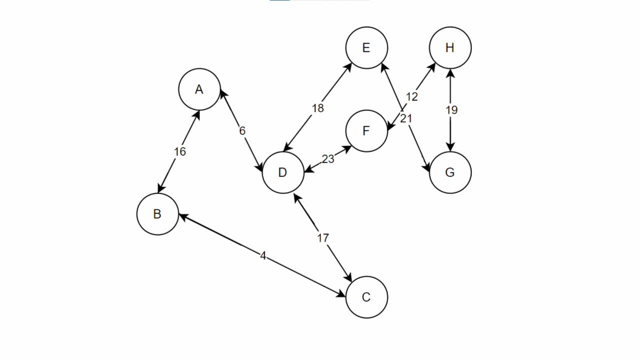 Wow, And now that we know a bit more about graph theory, we can start to build our postman's path. Let's start with a smaller neighborhood with just four intersections or vertices and four streets or edges, Seeing that each vertex has an even degree. 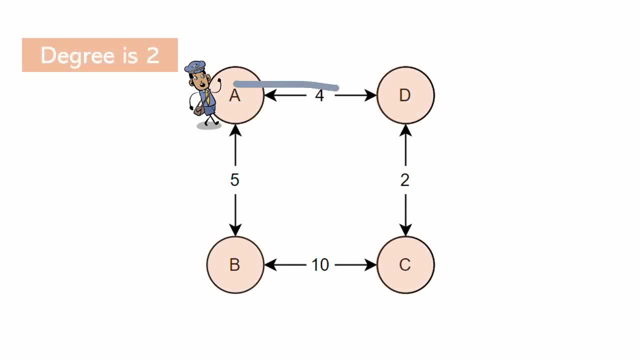 we know that the graph is Eulerian. From there we can quickly find the best path for our postman by just sketching out different paths until we find one that works. Knowing this route, our postman is able to quickly deliver the mail and rest for the night In this neighborhood. 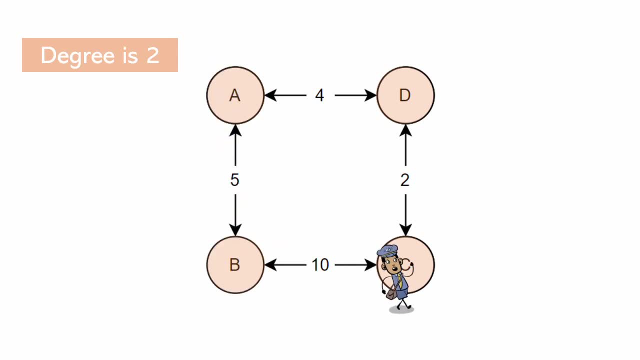 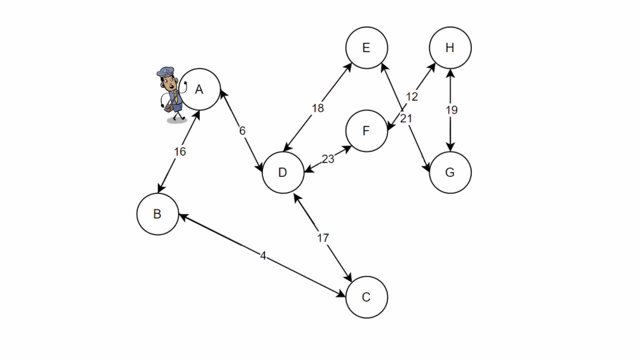 the postman can travel from the intersection A to B, to C to D and then back to A to traverse each edge. We can go back to our original neighborhood and use the same method to help our postman. From this we get the path A, B, C, D, E, G, H, F, D, A and the postman is able to complete the route quickly. 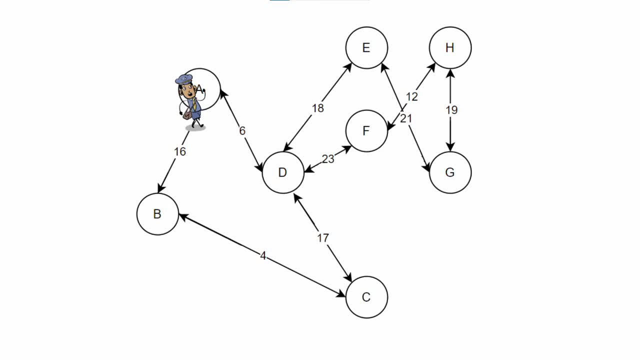 and rest for the night. This is just one of several paths which have the minimum weight of 136.. As long as the graph is Eulerian, there are more possible routes for our postman. The next day, the postman has to deliver the mail in a different neighborhood. 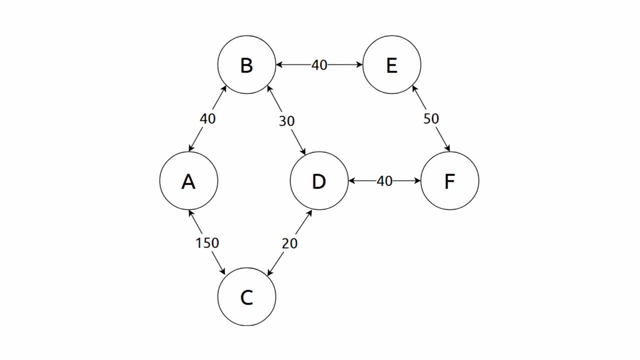 We already know that if the graph is Eulerian, we can easily find a route for the postman. But we count the degrees of each vertex and find that two of the vertices have odd degrees. What do we do now? Unfortunately, not all neighborhoods will be Eulerian. Sometimes our neighborhood is. 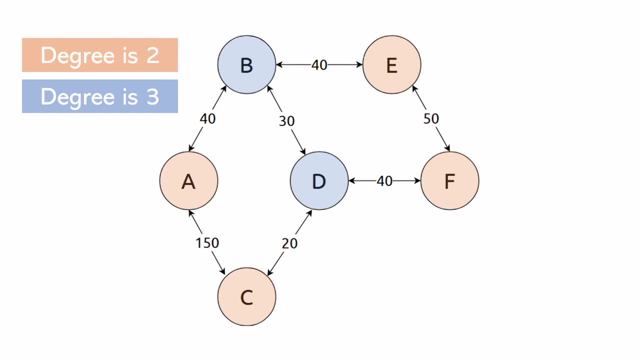 semi-Eulerian with two vertices of odd degree, so we'll have to repeat some edges. But also, since it's semi-Eulerian, we only have to repeat the path between the two vertices of odd degree. Think of it as adding an extra edge between those two odd vertices. With this extra edge each of. 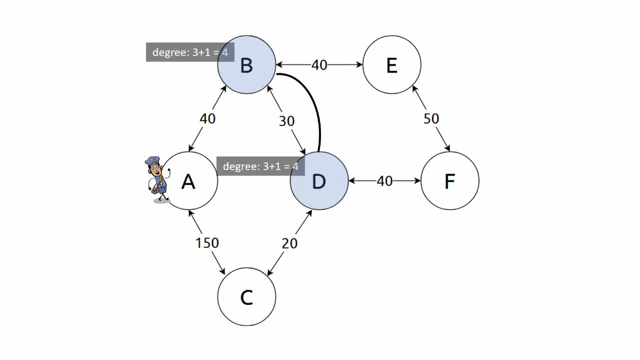 these vertices' degrees increase by 1, thereby making those values even. And now, since all the vertices will have an even degree, we can create an Eulerian path. In this scenario, the postman can go from A to B to D, to F to E to B, to D, to C to A. This path has a distance of 370 meters. 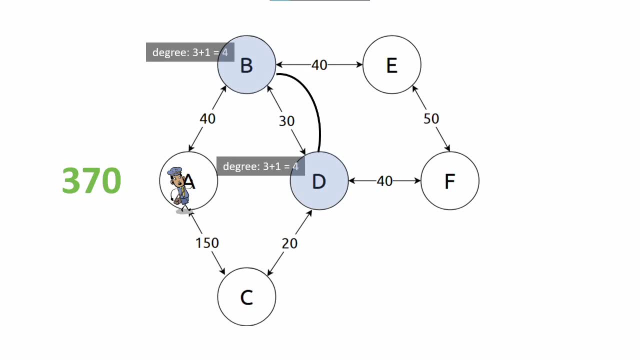 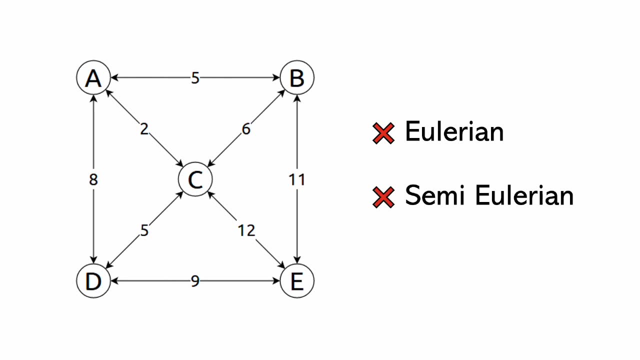 Ok, so after delivering the mail in the semi-Eulerian neighborhood, our postman moves on to the next one. Sometimes we are in a neighborhood like this one that neither has an Eulerian nor a semi-Eulerian graph, so we'll have to. 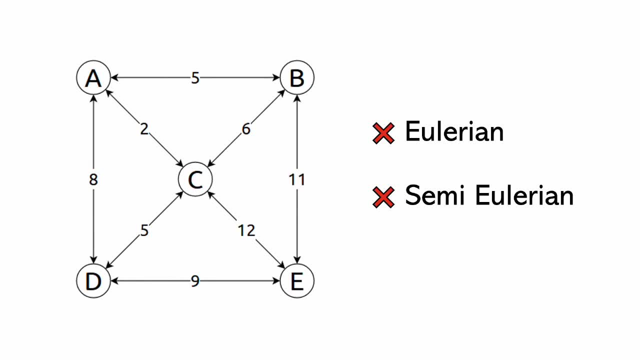 be more careful about how we minimize the weight of the root we take. Similar to our method in the last neighborhood, we can reduce the workload by finding the shortest possible roots between all the vertices of odd degree. That's right. Let's first identify all the vertices of odd degree. We can write this: 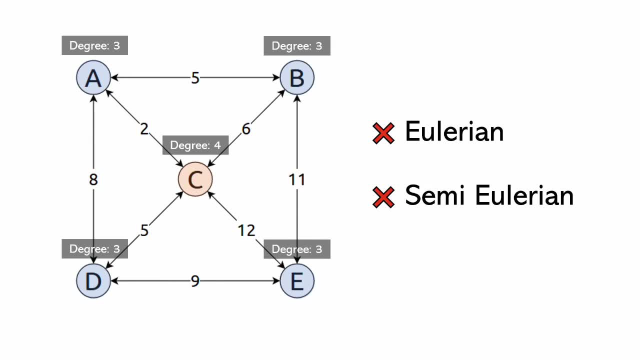 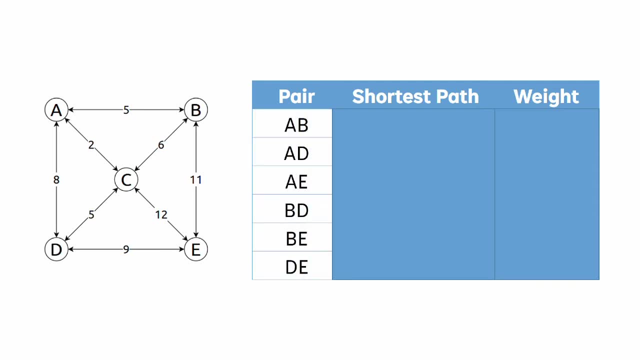 in a chart. Then, since the postman is traveling on the edges, we want to find the shortest root between all the vertices. We can start by writing out all the pairings of the start and end vertices. Going down the list, we can identify the shortest root and make note. 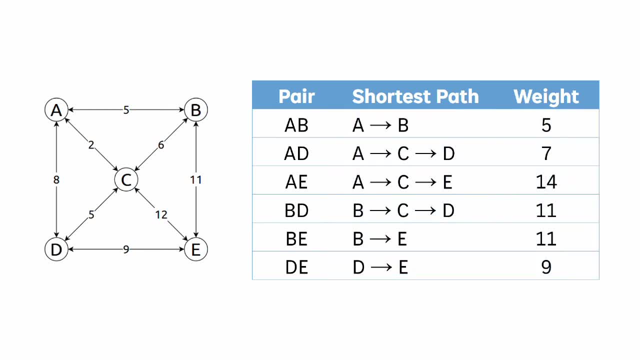 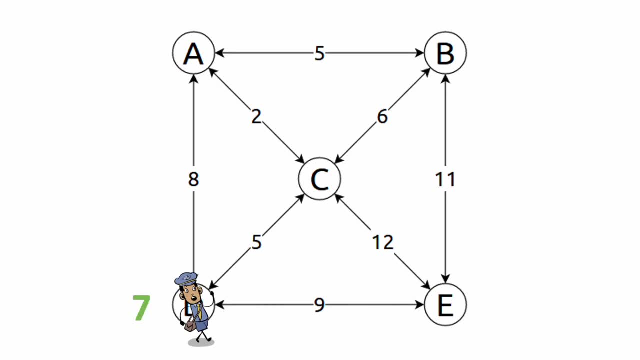 of the weight in the path we took. Oh, so for example, in this neighborhood to get from A to D, the shortest root is actually by going from A to C to D with weight of 7.. This is shorter than going directly from. 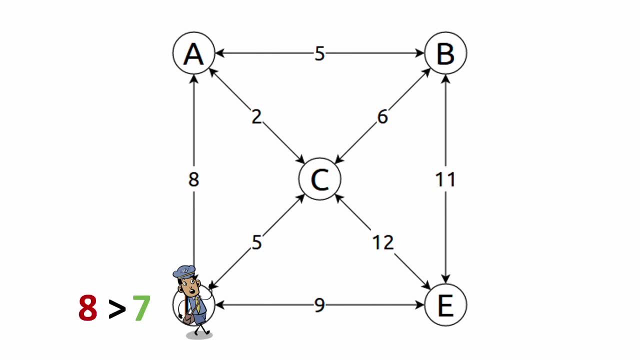 A to D, which has a weight of 8!. Yup, After completing the chart, we'll repeat the combination of the shortest pairings that will be taken. Yes, After completing the chart, we'll repeat the combination of the shortest pairings that. 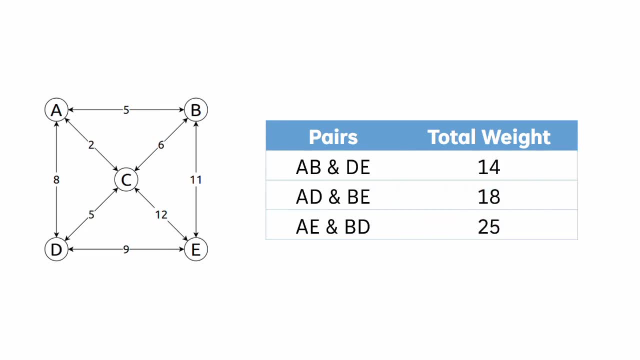 would get us through all the odd vertices which are AB and DE, And since we need to go on every street, we can find the weight of all the edges. then add on the combination of the shortest pairings yielding the shortest root. With this information, we can find the. 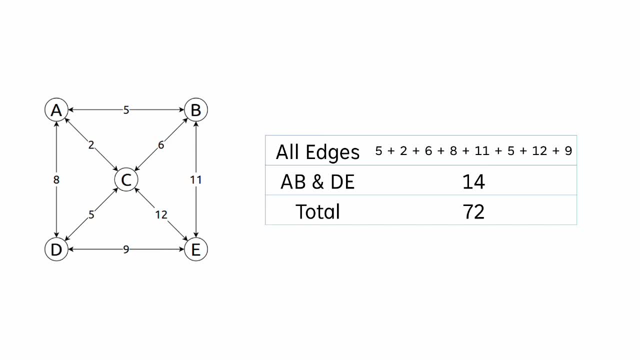 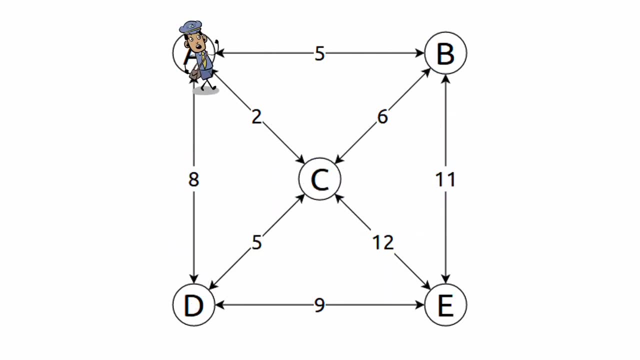 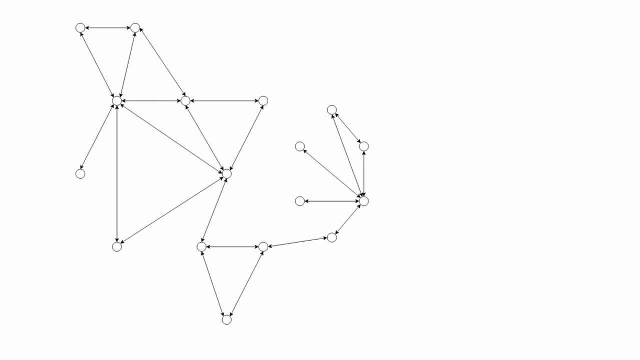 shortest path throughout the entire neighborhood and it's an easier day for the postman. For example: ABA, CBE, CDE, DA. What about a bigger neighborhood, town or city In larger neighborhoods? it would be easier to use the chart method, since manually inspecting different possible routes would take a millennium. 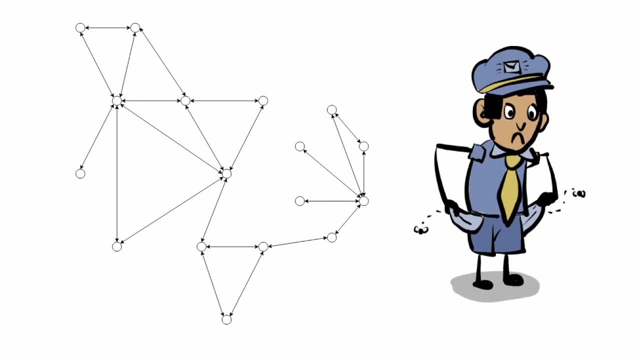 and our postman would run out of life savings. Instead of manually drawing out each path, it would be easier to find the shortest path between the vertices. So how would we solve it? for even larger scenarios, We can implement the chart method by using technology to find these graphs. The basic 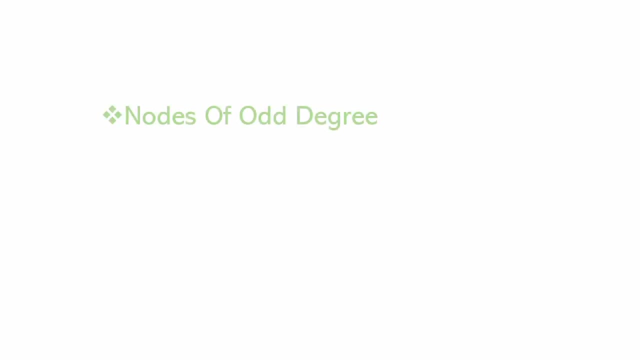 steps for doing this. have us find the nodes of odd degree, find the minimum distance pairs, compute the shortest paths between the vertices and find the shortest path. We can also use the chart method to find the shortest path between the node pairs and the minimum weights.